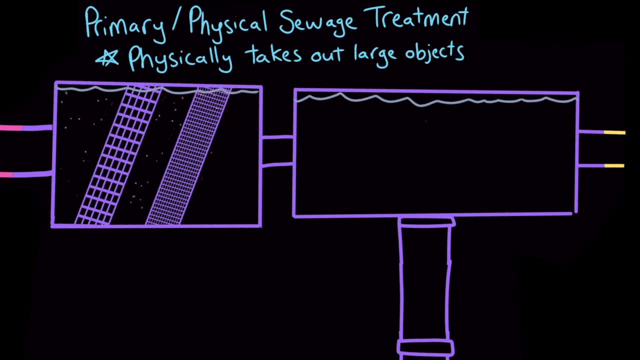 This prevents the objects from clogging up the pipes and pumps in future treatment steps. During primary treatment, the water goes through a series of screens that are progressively smaller and smaller openings. The screens sift out objects like sticks, rocks, rags, plastic bottles and Rubix's hair. 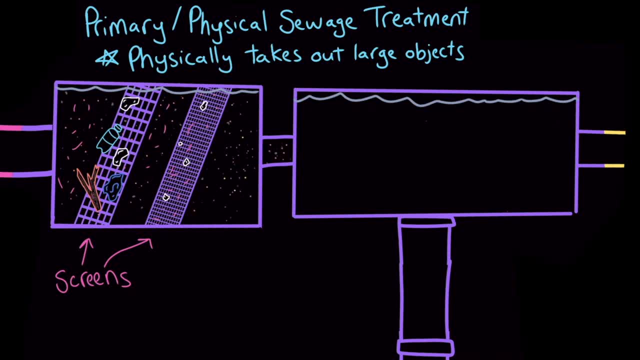 Even though the screens take out many of the larger objects, there's still a lot of grit in the water afterwards. Grit is made up of small loose particles of sand, gravel, coffee grounds, food waste and other pieces of material. To get rid of the grit, the treatment plant pumps 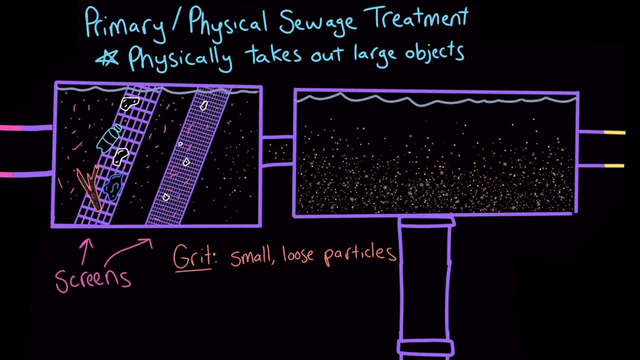 the water through long, narrow tanks that slow down the flow enough that the grit has time to settle to the bottom. All that thick, soft mud that gathers at the bottom of the grit tank is called sludge, and it's collected and treated. The water then moves on to secondary 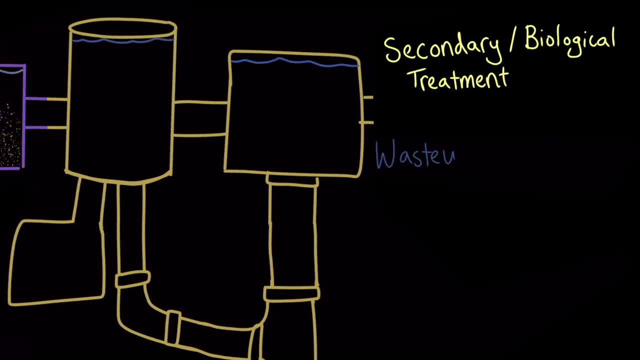 or biological treatment. During this stage, the wastewater is aerated or mixed with air to create perfect conditions to help increase the population of aerobic bacteria. Aerobic bacteria are important because they quickly feed on and break down the organic waste in the water. Sometimes bacteria-loaded sludge, called activated sludge, is used to. 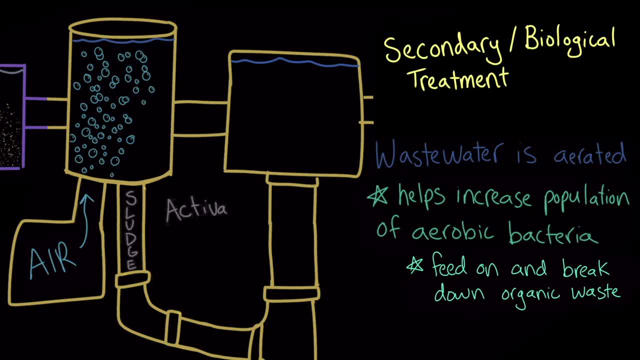 reduce the amount of organic waste in the water. Sometimes, bacteria-loaded sludge is also added to help grow even more bacteria. When the bacteria have plenty of oxygen, they metabolize the organic material into carbon dioxide. And, yes, more sludge, The sludge again. 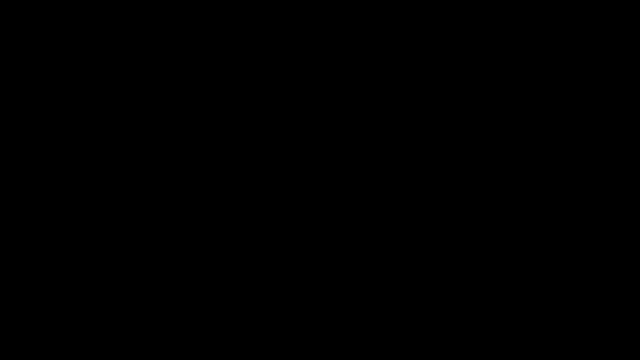 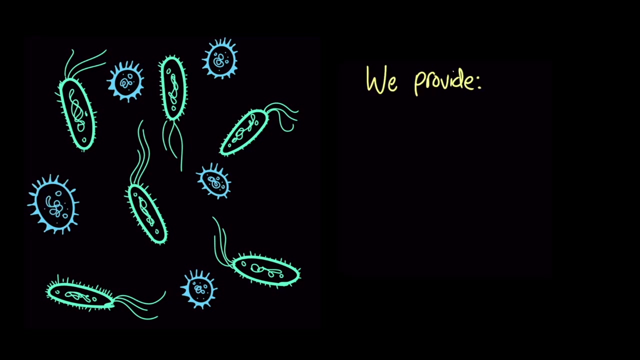 settles to the bottom of the tank and is collected for treatment. I like to think of secondary treatment as kind of like being a good caretaker to millions of microbial pets. When we provide our microscopic pets with oxygen and food, then they help us out by doing the. 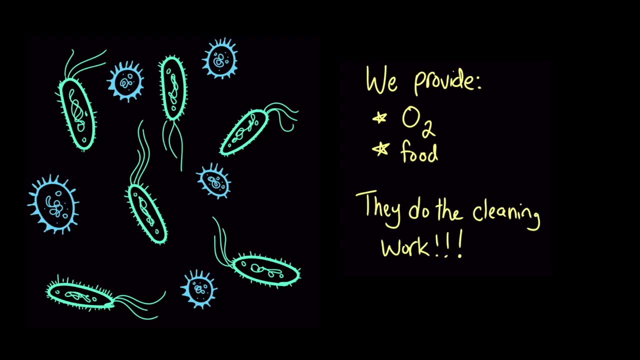 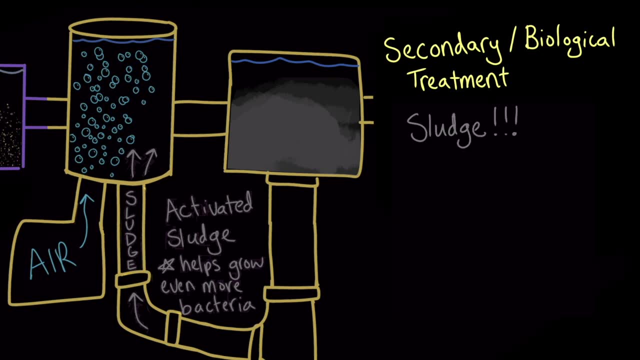 cleaning work. That's why secondary treatment is also called biological treatment, because it uses living organisms. Like primary treatment, secondary treatment generates lots of sludge. Some of the sludge may be recycled and added to water entering secondary treatment. This increases the population of aerobic bacteria in the wastewater, so the bacteria remove the 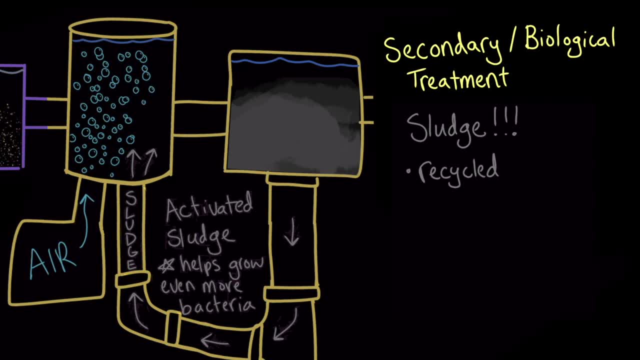 organic waste faster. The sludge collected from primary and secondary treatment can be dried and buried as a waste product or dehydrated and heated to make a soil-like material called biosolids that can be used in agriculture. By the time the primary and secondary treatment